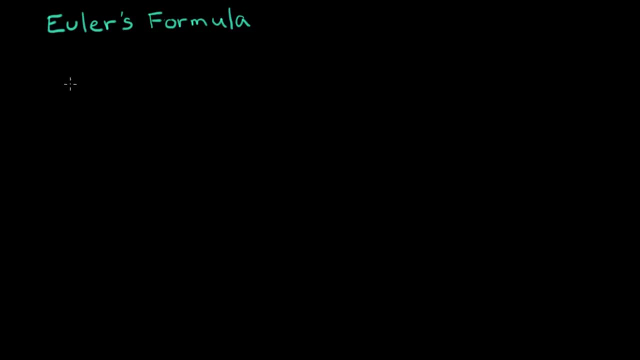 So in this video we're gonna talk about Euler's formula, and one of the things I wanna start out with is: why do we wanna talk about this rather odd-looking formula? What's the big deal about this? And there is a big deal, and the big deal is E. 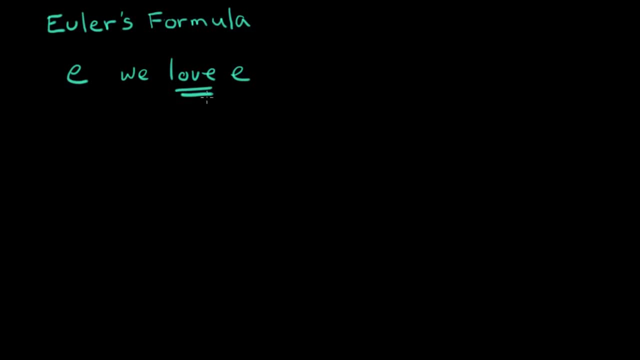 We love E And I'll underline that twice Now. the reason is because when we take a derivative of E, d dt of e to the x, equals e to the x And d? dt of e to the ax. so where a is anything? 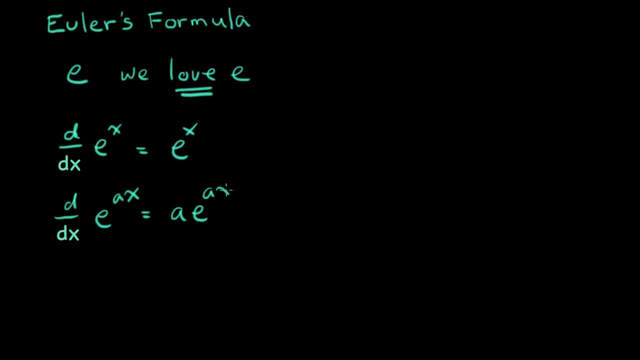 equals a e to the ax, And so the property is that when you take a derivative of the function, the same function comes out, Or if you take a derivative of the function, a scaled version of the same function comes out. And we love this because why? 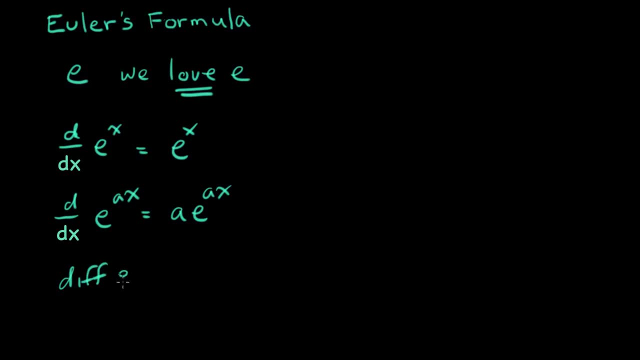 Because when we do differential equations, e to the x is the solution. Almost every time whenever we did a circuit, e to the x was the answer. If you recall from when we were solving circuits, simple circuits with differential equations, that we always said something like: 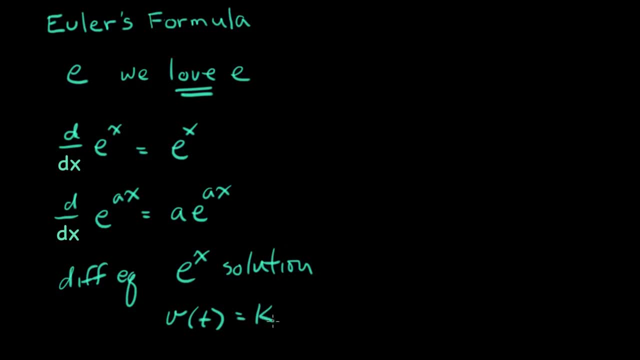 well, we're gonna guess that v of t is some constant times. e to the s? t. That was a proposed solution. This turned out to work every time, So there's something else we love too, And that is sinusoids, Or sines and cosines. 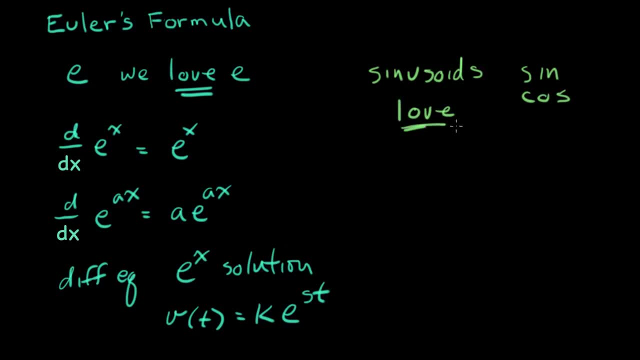 Okay, We love these, And that gets two lines. Now, why do we love these? It's because they happen in nature. They happen in nature. If you whistle, the air pressure looks like a sine wave. If you ring a bell: 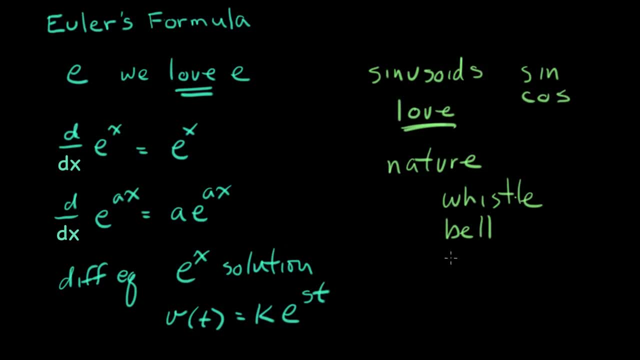 the bell moves in a sine wave, Any kind of music. if you look at the notes in music, the sound they make, the pressure waves look like sine waves And circuits make sine waves. Remember, we analyzed this circuit in great detail. 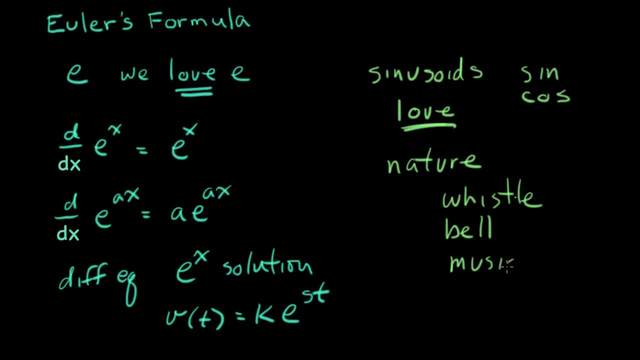 Any kind of music. If you look at the notes in music, the sound they make, the pressure waves look like sine waves And circuits make sine waves. Remember, we analyzed this circuit in great detail. It was the L C circuit. 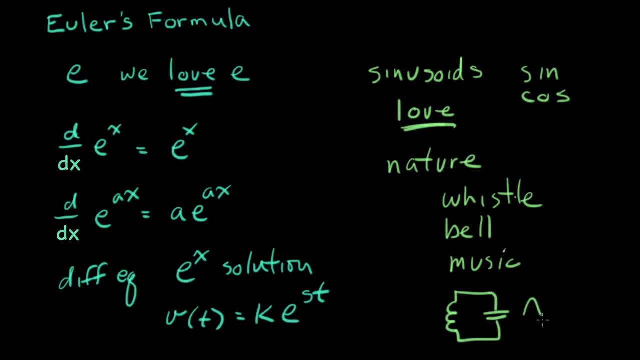 We looked at the natural response of this and that was a sine wave. Okay, so electric circuits make sine waves, All these things make sine waves. They occur in nature And we wanna be able to analyze things that happen when sine waves are present. 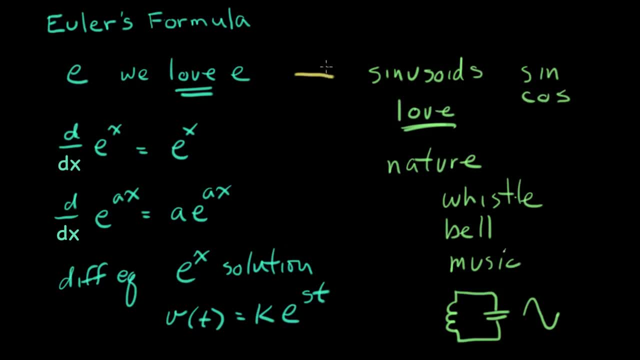 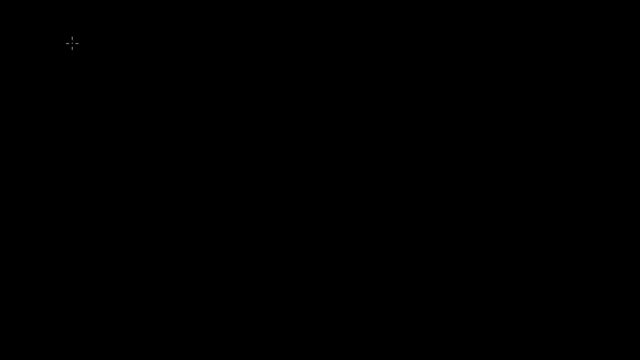 So we have two things we love And we wanna relate these two things And these are gonna be related through that Or there's formula That's how we connect these two separate ideas, And let's go do that. So Euler's formula says that: 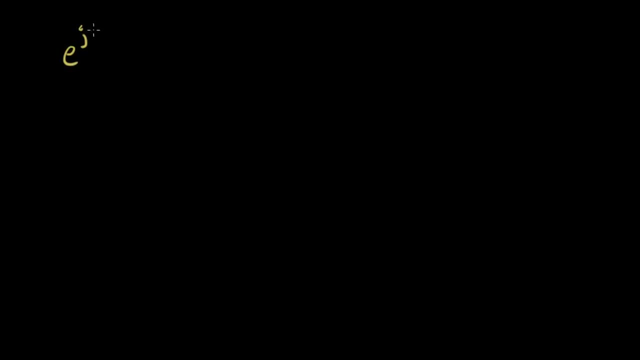 E to the J X equals cosine X plus J times sine X. Now Sal has a really nice video where he actually proves that this is true, And he does it by taking the McLaurin series expansions of E and cosine and sine and showing that this expression is true. 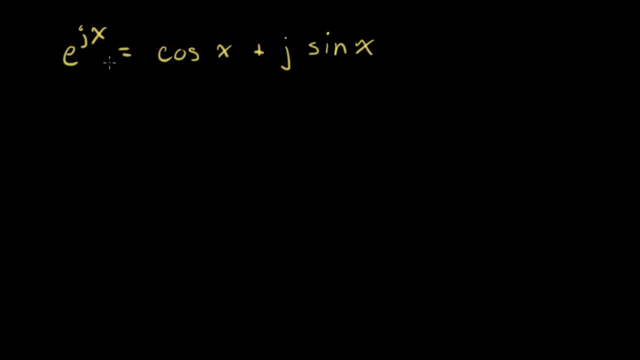 by comparing those series expansions. Now, I'm not gonna repeat that here, We're just gonna state that as fact And now we're gonna look at this equation a little bit more. So this is the expression that relates exponentials that we love. 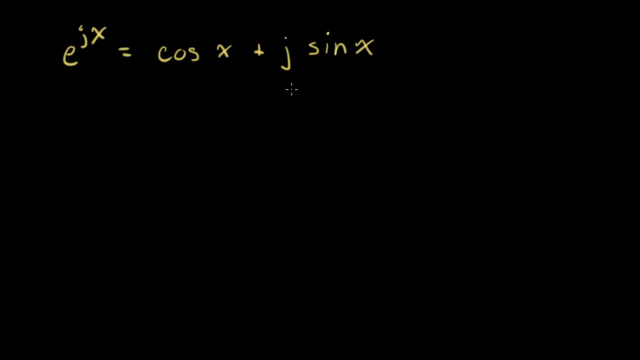 to sines and cosines that we love, And part of the price of doing that is we introduce complex numbers into our world. Here's two complex numbers. Okay, this is where complex numbers come into electrical engineering. So I have to mention the other form. 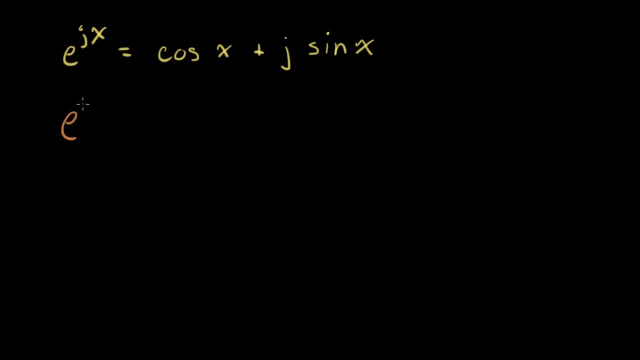 of this formula, which is E to the- I put a minus sign in here- E to the minus J X, And that equals cosine X minus J sine X. So these two expressions together are Euler's formula, or Euler's formulas, And we're gonna exploit this by taking 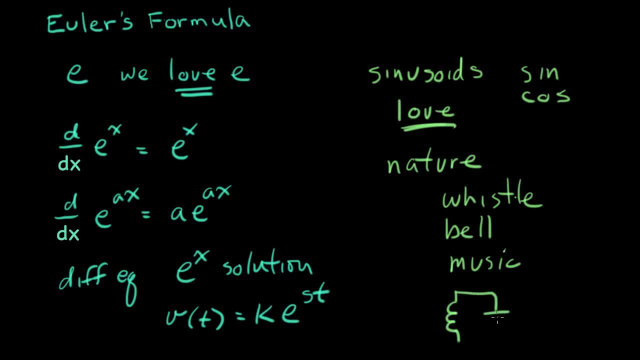 It was the L C circuit. We looked at the natural response of this and that was a sine wave. Okay, So electric circuits make sine waves. All these things make sine waves. They occur in nature And we wanna be able to analyze things that happen. 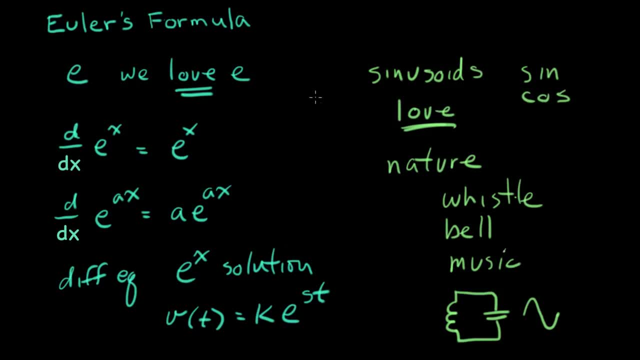 when sine waves are present. So we have two things we love And we wanna relate these two things And these are gonna be related through that Or there's formula. That's how we connect these two separate ideas And let's go do that. 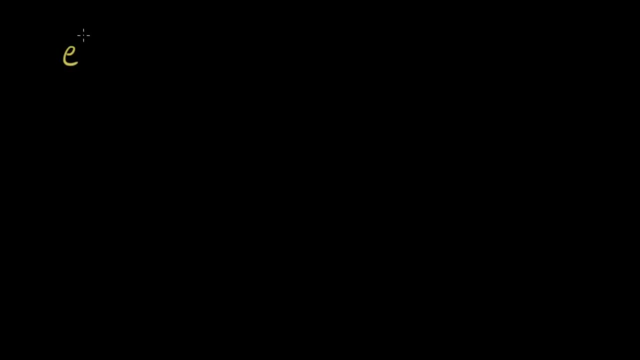 So Euler's formula says that E to the J X equals cosine X plus J times sine X. Sal has a really nice video where he actually proves that this is true, And he does it by taking the Maclaurin series: expansions of E and cosine and sine. 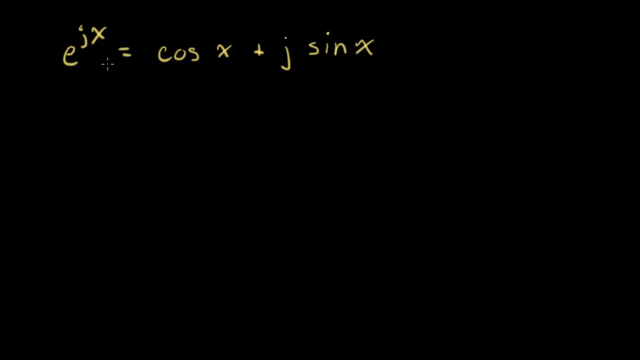 and showing that this expression is true by comparing those series: expansions. Now I'm not gonna repeat that here, We're just gonna state that as fact, And now we're gonna look at this equation a little bit more. So this is the expression that relates exponentials that we love. 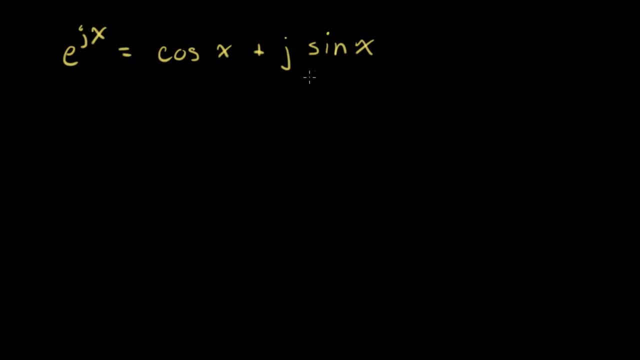 to sines and cosines that we love, And part of the price of doing that is we introduce complex numbers into our world. Here's two complex numbers. Okay, this is where complex numbers come into electrical engineering. So I have to mention the other form of this formula. 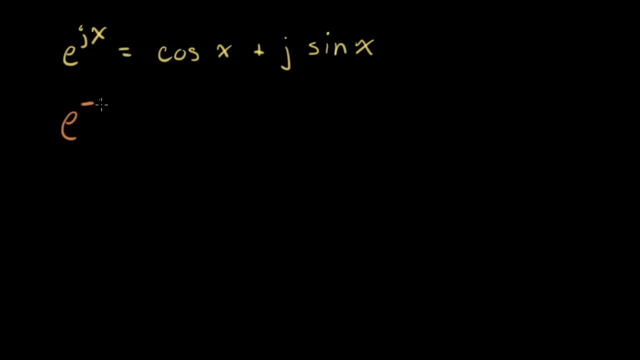 which is E to the- I put a minus sign in here- E to the minus J X, And that equals cosine X minus J sine X. So these two expressions together are Euler's formula, or Euler's formulas, And we're gonna exploit this by taking 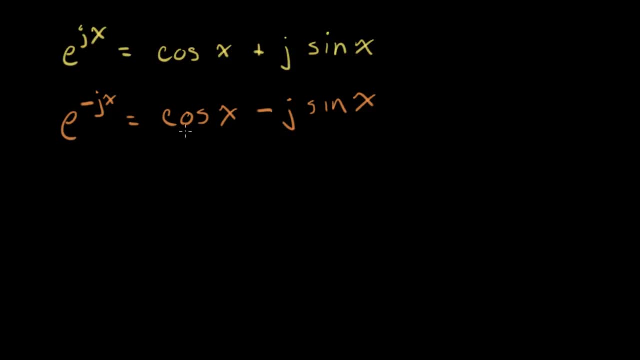 we'll be able to take the cosines and sines that we find in nature. We're gonna be able to fashion them into exponentials And these exponentials then go into our differential equations and give us solutions, And we're gonna come back and pull out. 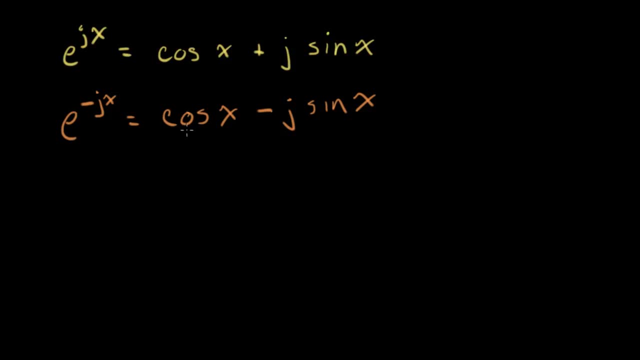 we'll be able to take the cosines and sines that we find in nature. We're gonna be able to fashion them into exponentials And these exponentials then go into our differential equations and give us solutions, And we're gonna come back and pull out. 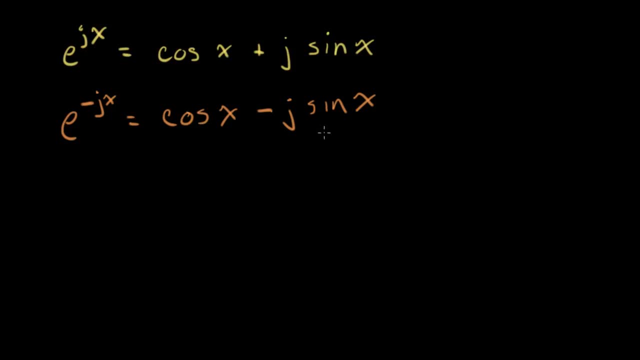 the cosines and sines. That's the rhythm of how we're gonna use this equation to help us solve circuits. One small point I wanna share: Notice that in both these equations the cosine comes first and the sine is over here, on the imaginary side. 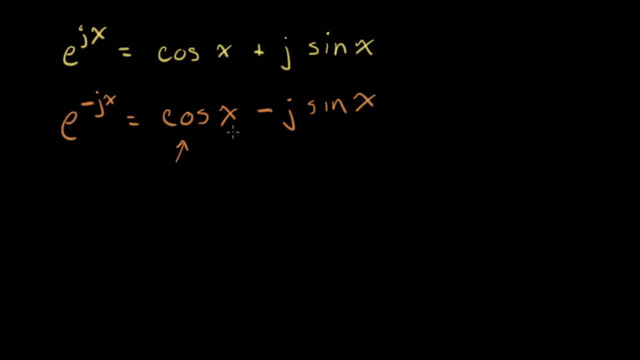 So the cosine is on the real side. This is the reason that we have a preference. in the future, We're gonna have a preference for talking about our real world signals in terms of the cosine function. It's because, in this Euler's formula, 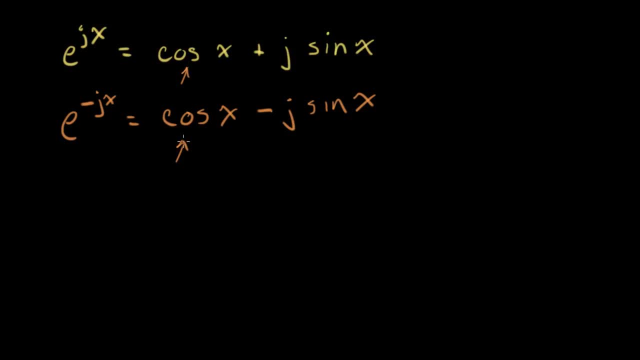 the cosine comes first in both cases. So what I wanna do now is take a second, and I wanna see if we have any. if we had our signal expressed in these exponentials, how do we recover the cosine and the sine term? How do we flip these equations around? 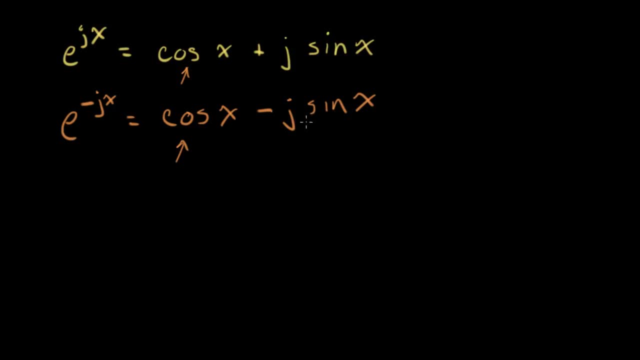 so we can solve for the cosine and the sine. It's a simple bit of algebra here. It's good to see, Alright, so if I wanna isolate the cosine term, if I wanna isolate the cosine term, let me get rid of these guys here. 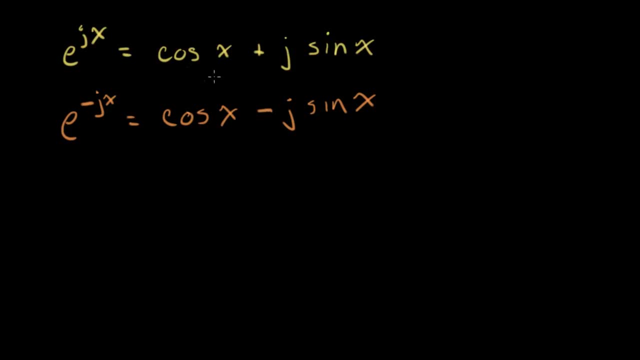 So now to isolate the cosine term, what I'm gonna do is add these two equations together and that plus and minus are gonna cancel out this second term here. That's what I'm going for. So if I add, I'll get e to the jx. 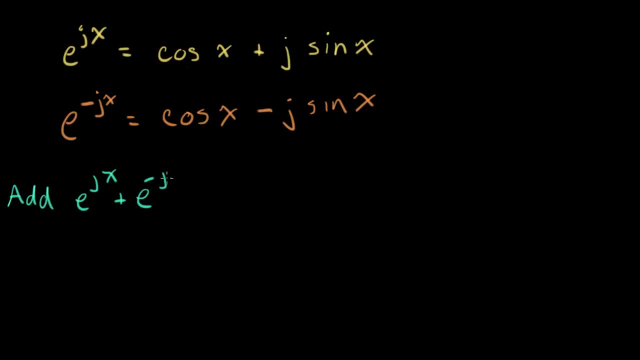 plus e to the minus jx equals cosine doubles two, cosine x and the two sine terms cancel out right. So then I can write. I'll write it over here. I can write: cosine of x equals e to the plus jx, plus e to the minus jx. 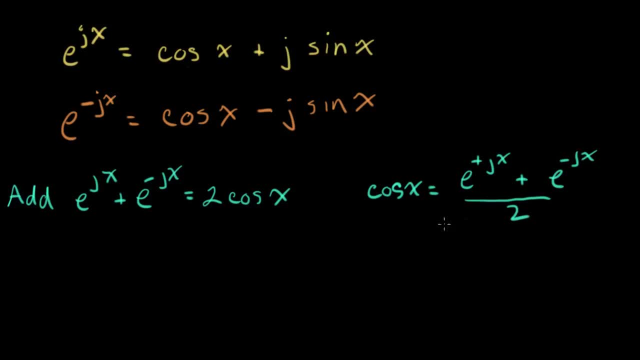 over two. Alright, so that's the expression. that's the expression for cosine in terms of complex exponentials. Okay, let's go back and see if we can get sine. So what I'm gonna do with sine is I'm gonna subtract. 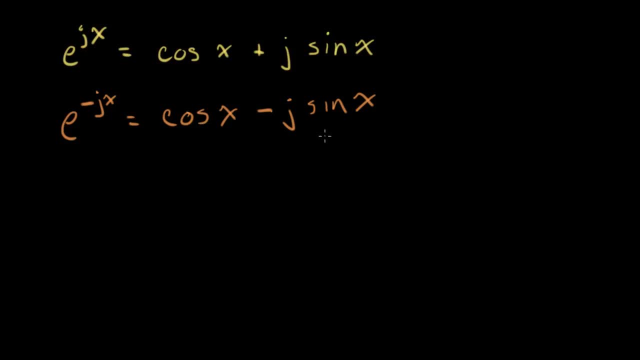 the cosines and sines. That's the rhythm of how we're gonna use this equation to help us solve circuits. One small point I wanna share: Notice that in both these equations the cosine comes first and the sine is over here, on the imaginary side. 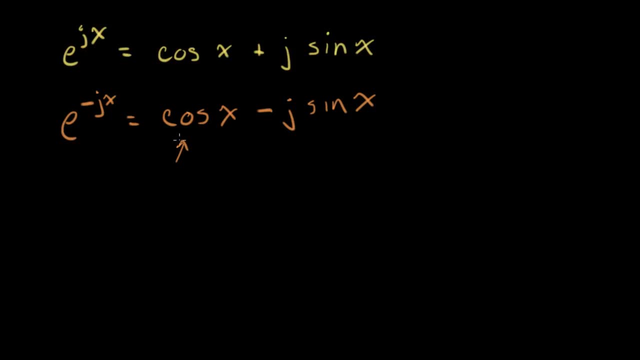 So the cosine is on the real side. This is the reason that we have a preference. in the future, We're gonna have a preference for talking about our real world signals in terms of the cosine function. It's because, in this Euler's formula, 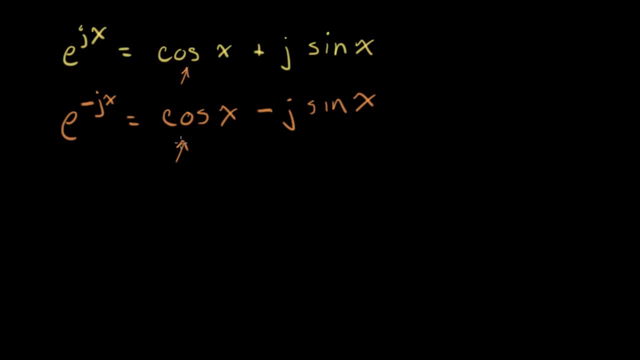 the cosine comes first in both cases. So what I wanna do now is take a second and I wanna see if we had our signal expressed in these exponentials. how do we recover the cosine and the sine term? How do we flip these equations around? 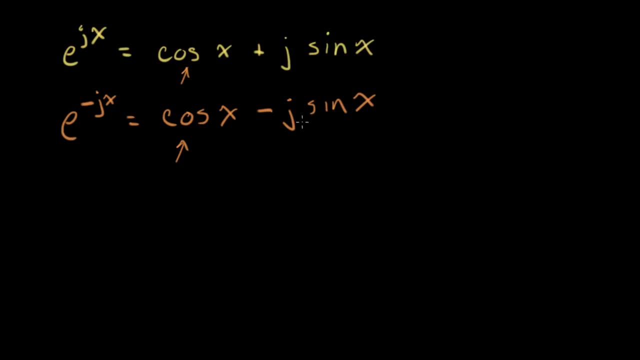 so we can solve for the cosine and the sine. It's a simple bit of algebra here. It's good to see, Alright, so if I wanna isolate the cosine term, if I wanna isolate the cosine term, let me get rid of these guys here. 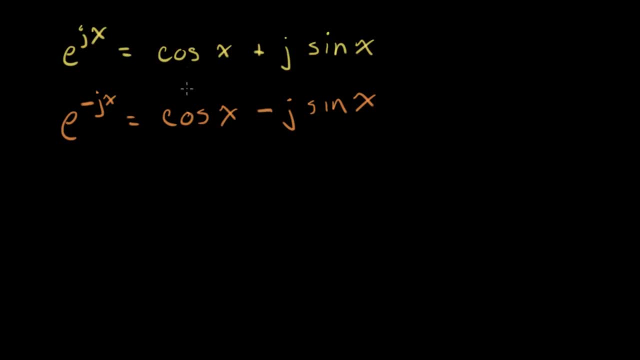 So now to isolate the cosine term, what I'm gonna do is add these two equations together and that plus and minus are gonna cancel out this second term here. That's what I'm going for. So if I add, I'll get e to the jx. 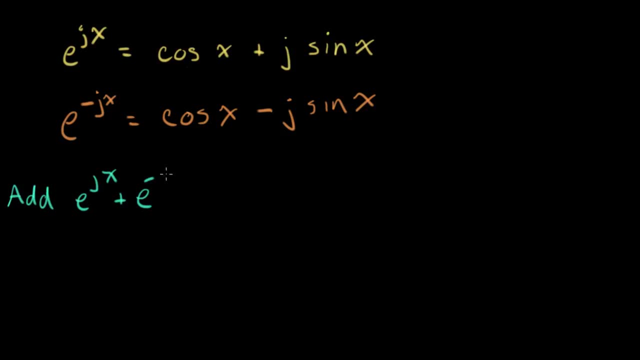 plus e to the minus jx equals cosine, doubles two, cosine x and the two sine terms cancel out right. So then I can write. I'll write it over here. I can write: cosine of x equals e to the plus jx. 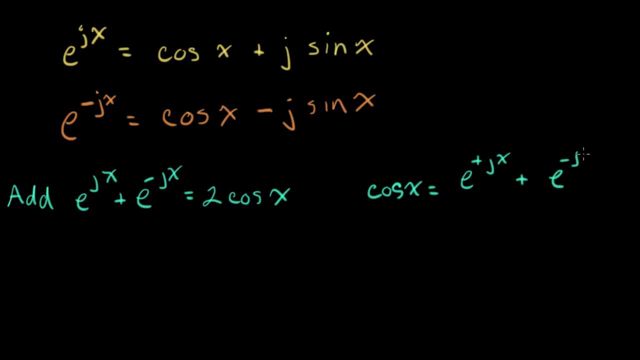 plus e to the minus jx over two. Alright, so that's the expression. that's the expression for cosine in terms of complex exponentials. Okay, let's go back and see if we can get sine. So what I'm gonna do with sine?